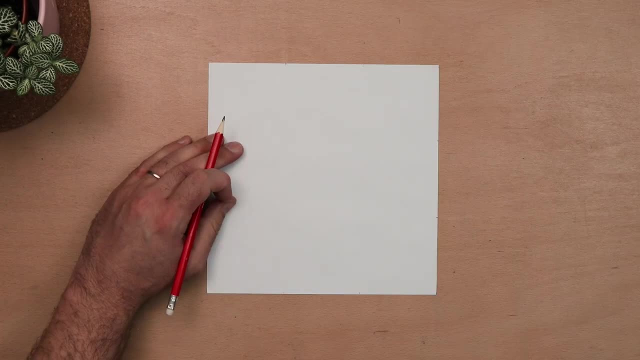 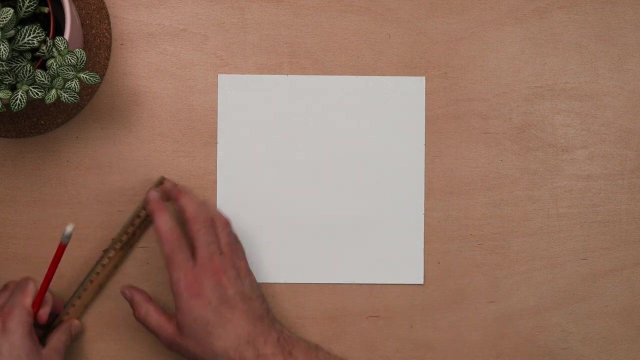 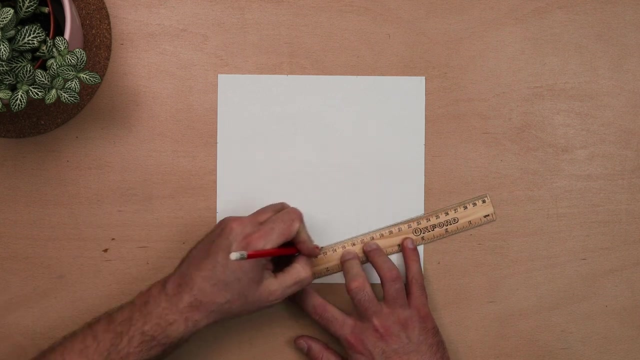 into your art activity. Choose one corner of the paper and draw straight lines from that corner to all the other marked points on the opposite sides of the paper. Now that sounds tricky, but it's really obvious when you start drawing. Oh, and remember to always draw to the opposite corner. that's important. 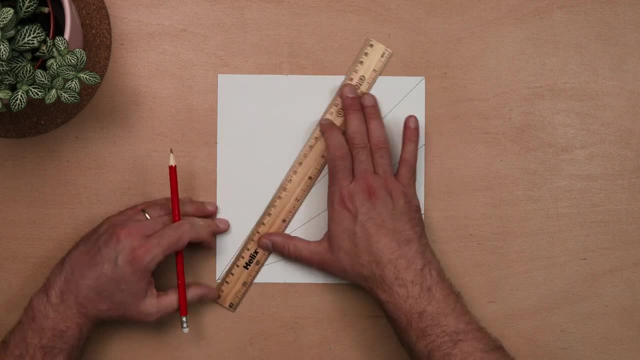 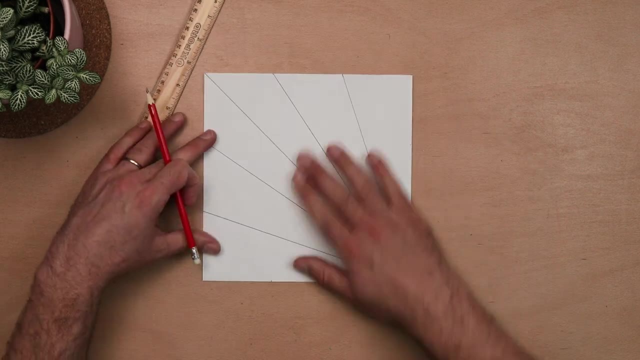 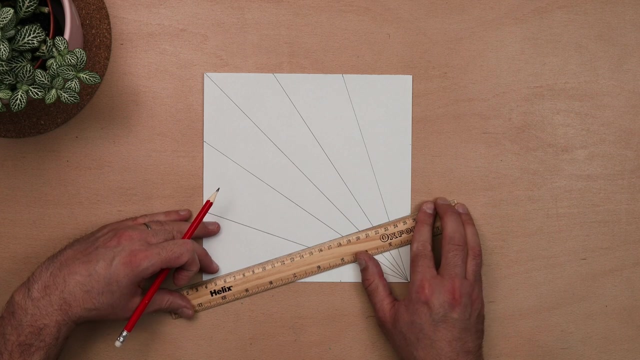 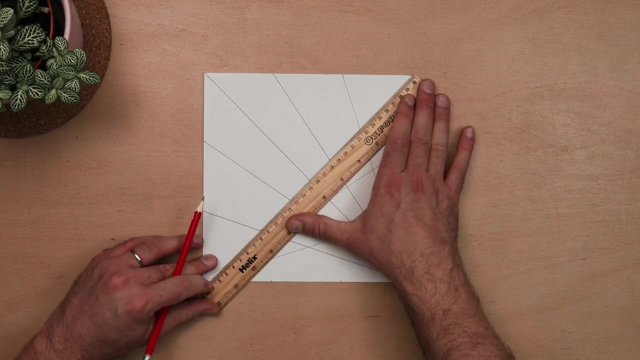 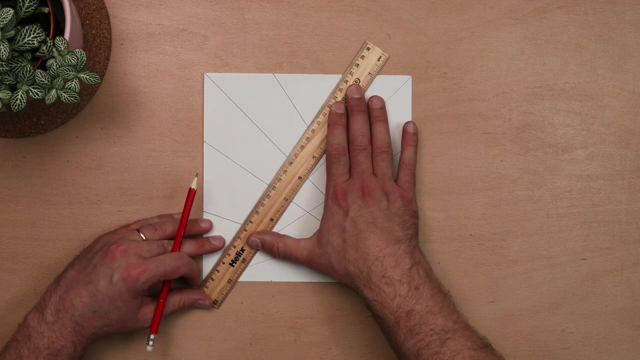 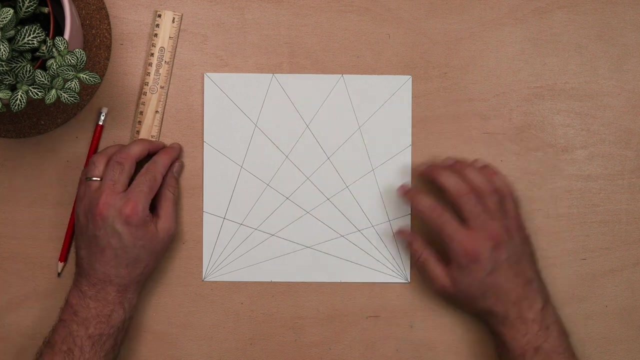 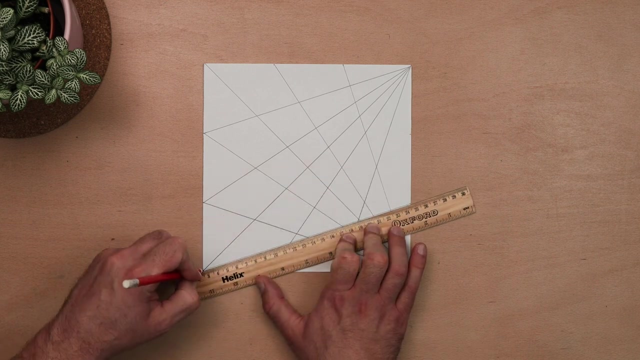 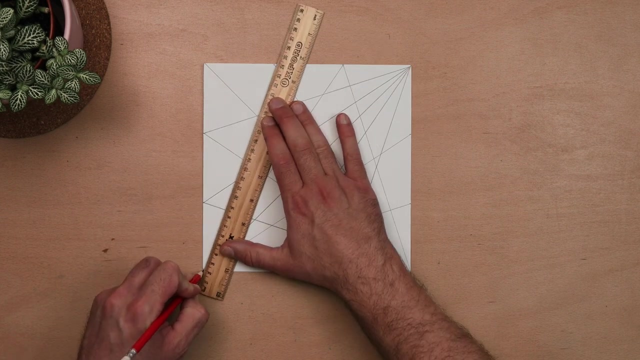 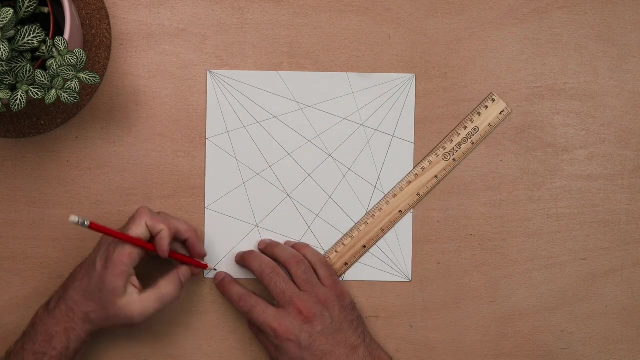 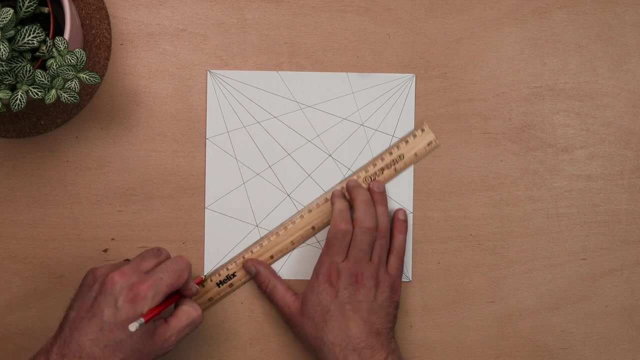 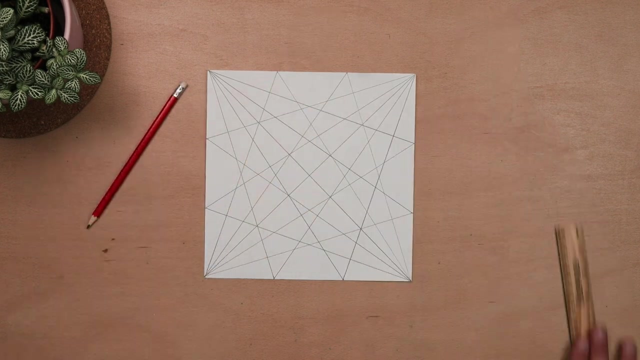 Once this is done, turn your paper and do the exact same with all the other corners. you now just choose a segment from one of the corners and shade it in with your pencil, and if you have color pencils or felt tip pens, that also looks better. 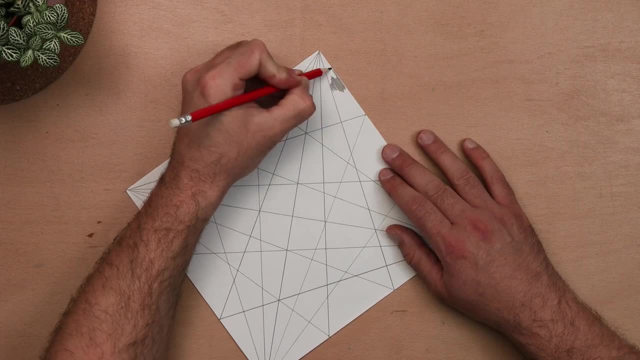 Now to fill in the corners, we're going to need a pencil and we're going to need a pencil. Now to fill in the corners, we're going to need a pencil and we're going to need a pencil. felt tip pens- that also looks good, but I like the metallic, shiny look of a. 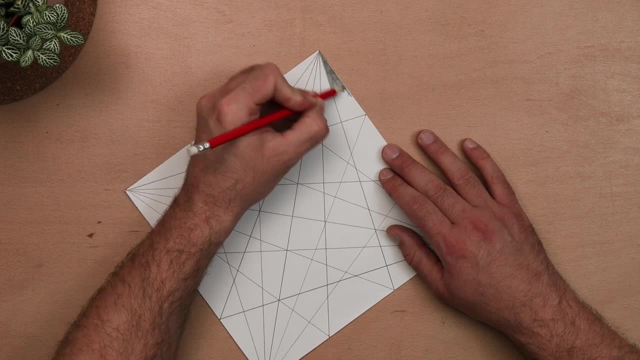 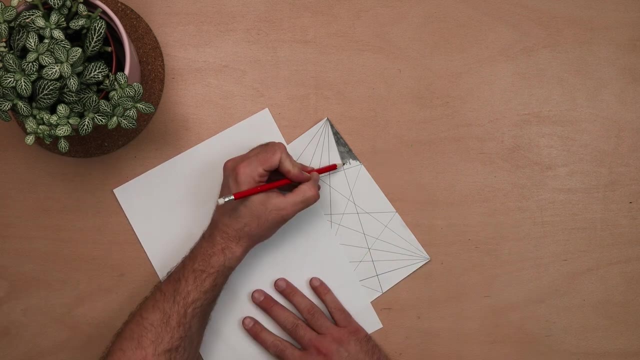 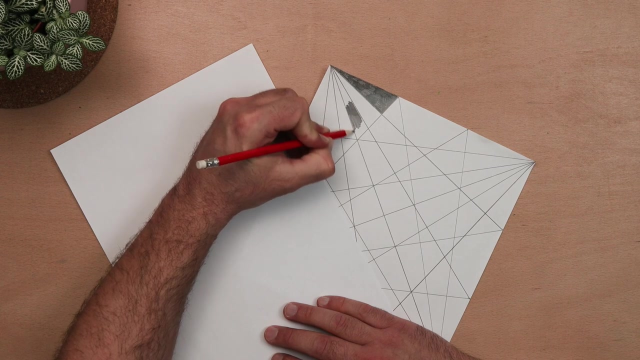 pencil. And here's a top tip: put a spare bit of paper under your hand to stop the pencil from smudging. Once shaded, skip a segment, then shade the next one. You want to keep a white segment in between so that no two shaded bits touch along their edge. 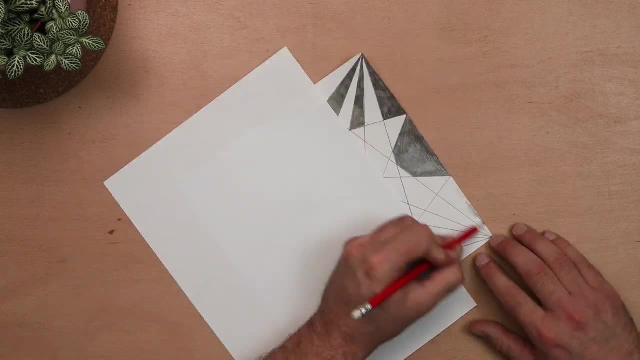 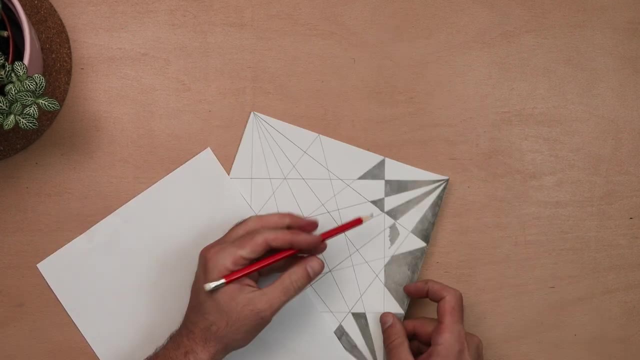 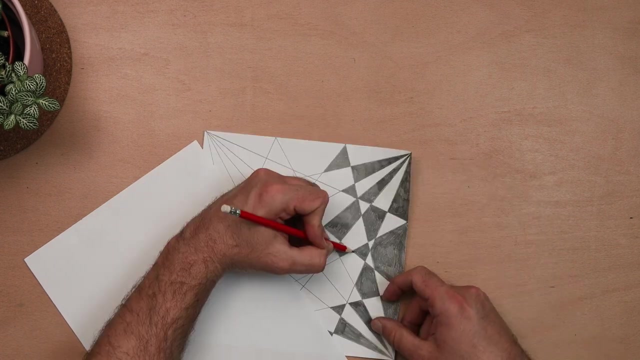 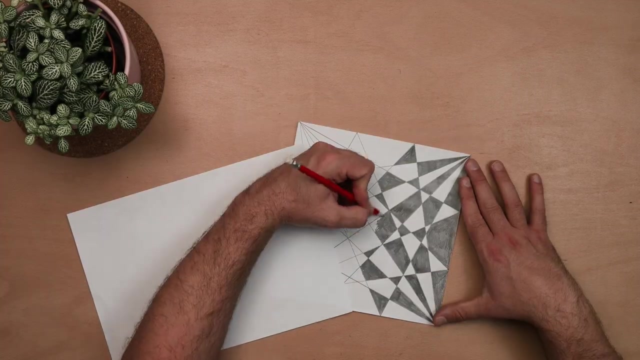 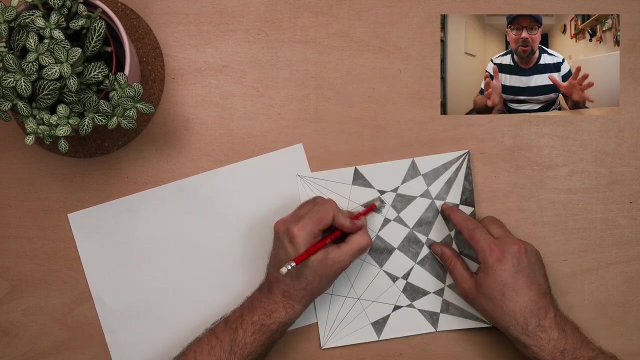 This will seem tricky at first, but it becomes very clear as you do it, especially as each corner is symmetrical: Up, close, up close, From the bottom Right. and remember you're short of time, which I imagine many of you are. you don't need to do this in one stitch. Instead, clip your pencil onto incident table, or two, such as this: